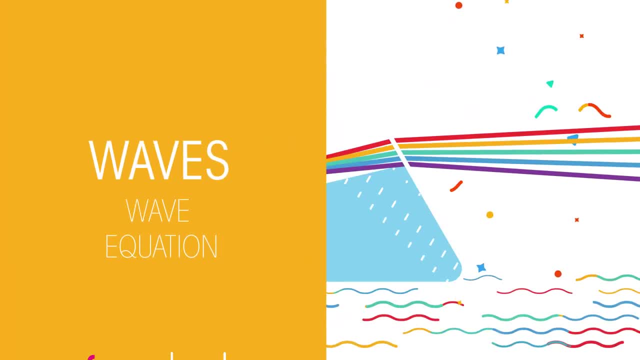 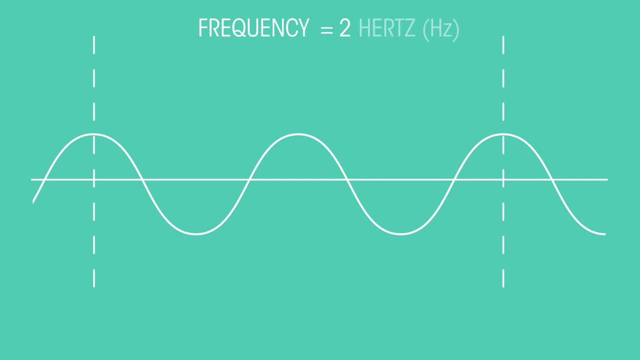 Waves have a frequency: the number of complete waves passing a point every second, and measured in hertz: Wavelength, the distance between two consecutive points on a wave. and amplitude: the distance of maximum displacement. both can range from a thousandth of a millimetre. 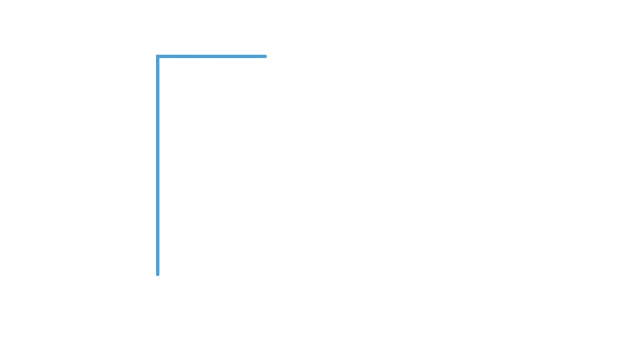 to hundreds of metres, which we looked at in this video. You may want to watch that first before we look at using these values in equations to calculate the speed at which they can travel. The frequency, wavelength and how fast the wave is travelling are all 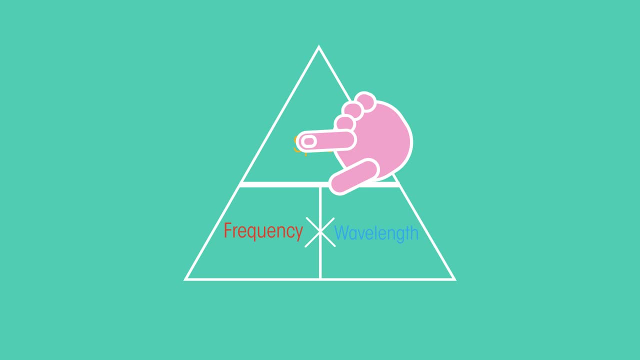 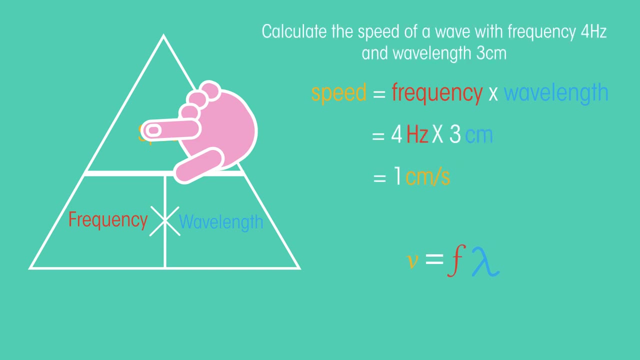 connected. If we want speed, we put our finger over speed, and it equals frequency times wavelength, which, in symbols, is this: We can use it to calculate the speed of a wave with frequency at 4 hertz and wavelength at 3 centimetres. Look at the units. The frequency is measured. 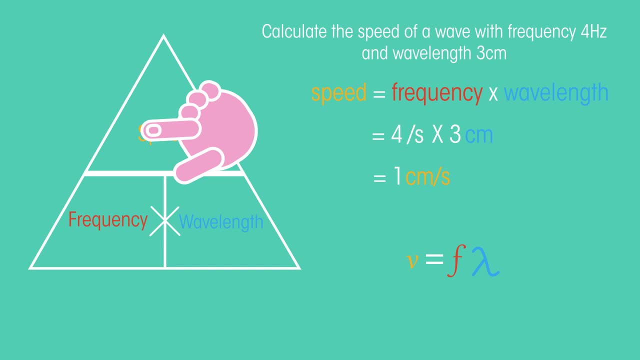 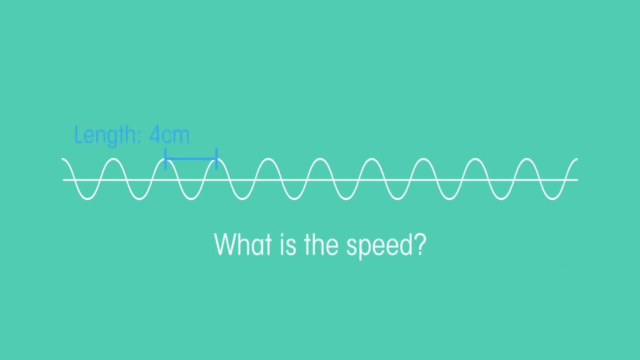 in hertz, which is a measure of per second, and the wavelength here is in centimetres, So the speed must be in centimetres per second. Let's have a look at another example. What speed is a wave travelling at if its length is 4 centimetres and its frequency is 10 hertz? 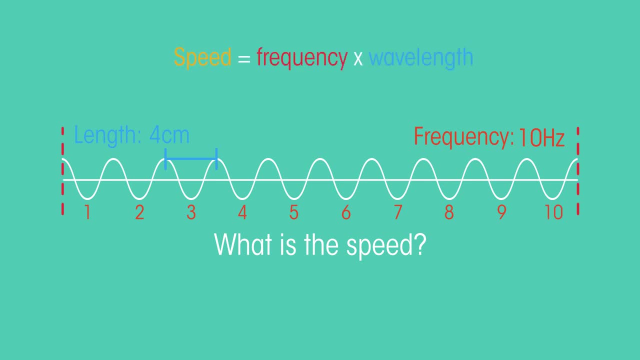 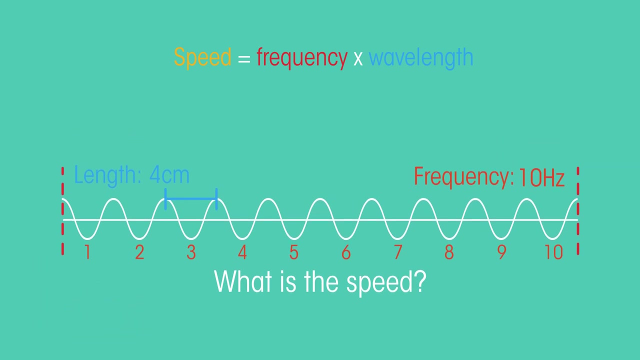 We will be using this equation, so we always need to start by writing it down and we just enter the values from the question. You give it a go. Think carefully about the units. pause the video, find the speed and click play when you're ready. 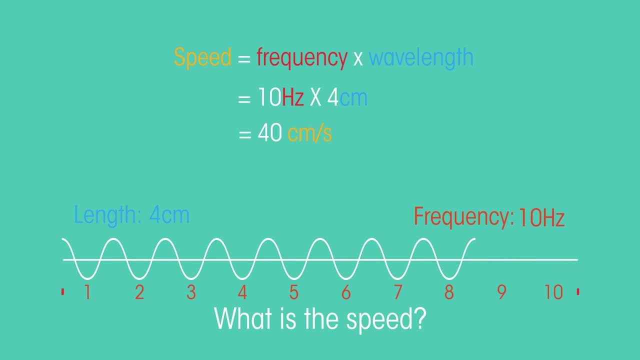 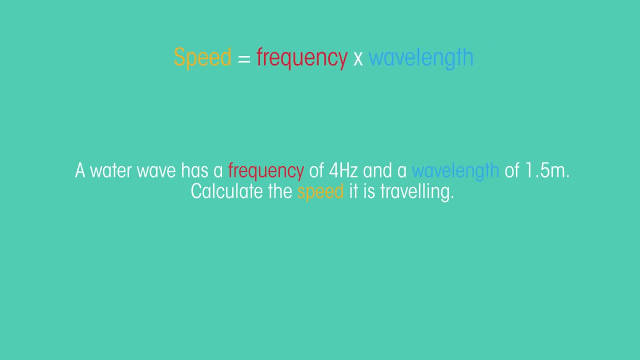 Did you remember that the hertz means per second, so the speed unit is centimetres per second. Here's another one for you to do. Remember to write down the equation first and check what units are being used. Pause the video, work it out and click play when. 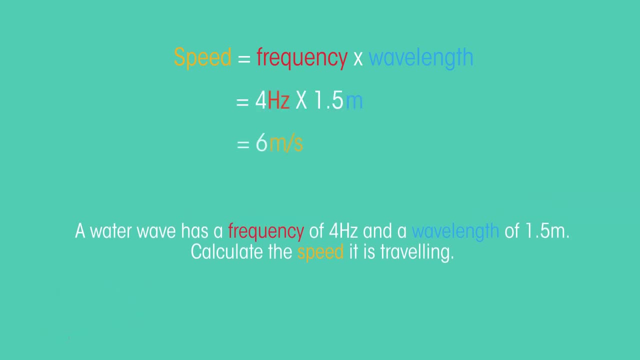 you're ready? How did you get on? Did you get caught out by the change in units? Here? the value for wavelength was measured in metres, and so our answer must be in metres per second. So far we've been calculating the speed, but we could just as easily be.